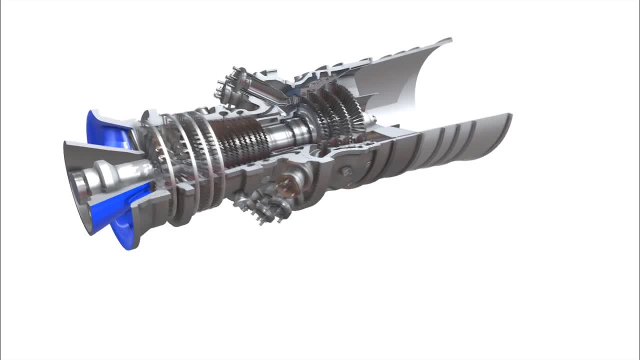 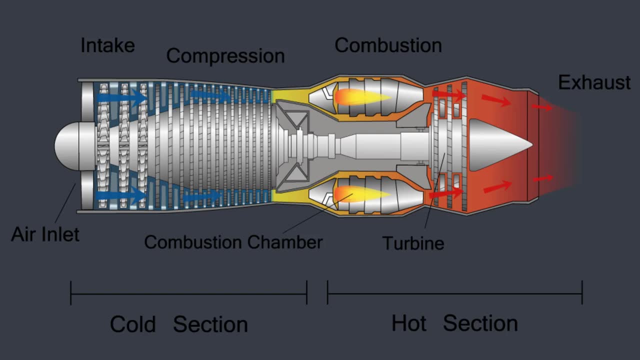 In this one I'm gonna take a look at something a little bit random. I want to take a look at a gas turbine. Gas turbines are also known as combustion turbines. They're used for power generation. They're used for pushing ships through the water. 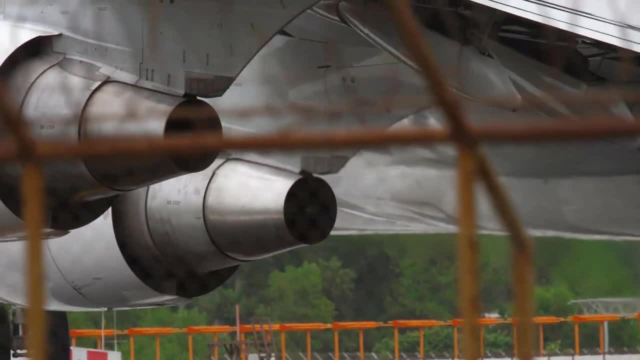 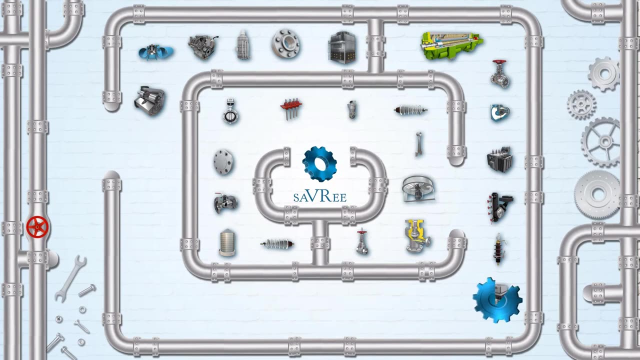 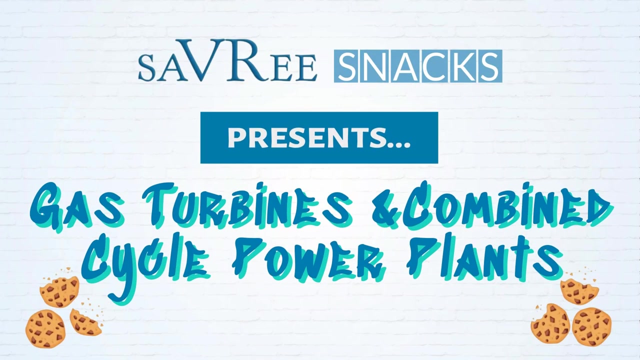 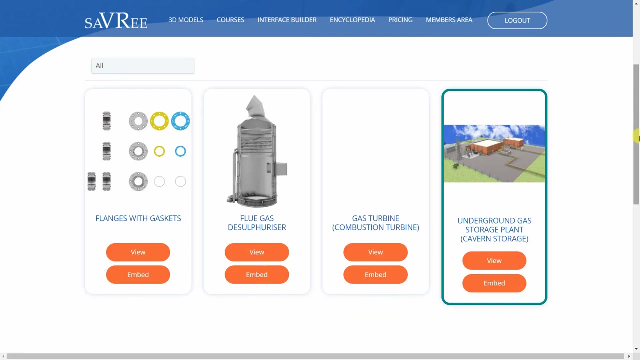 They're used for making aircraft fly. A pretty useful machine is a gas turbine. So let's have a look at a gas turbine. Go down here. Doesn't have an image yet because it's hot off. the press Only recently finished And here we go. 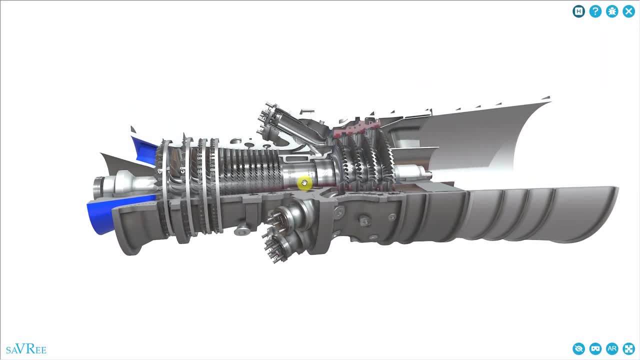 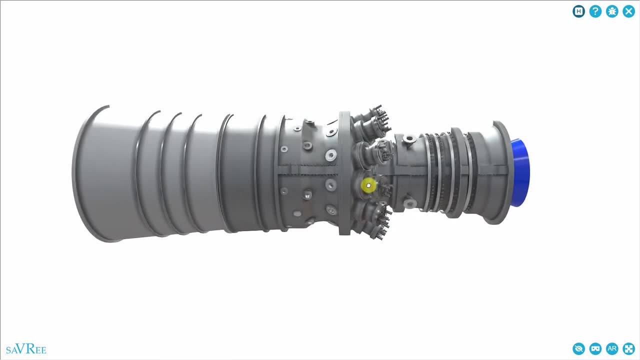 This is a gas turbine, also called a combustion turbine. There is no difference between the two terms. We go around here. You can see it from this angle. It's beautiful. It is a engineering wonder. believe me, I'll explain to you exactly how it works now. 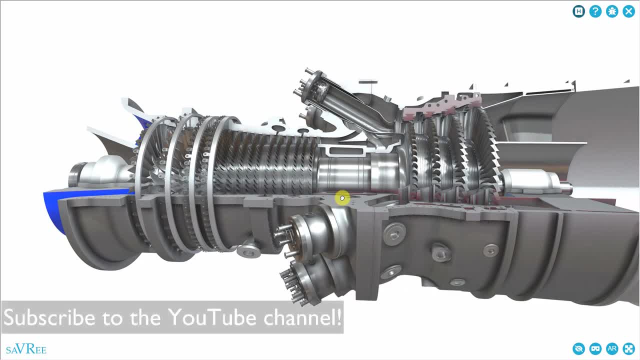 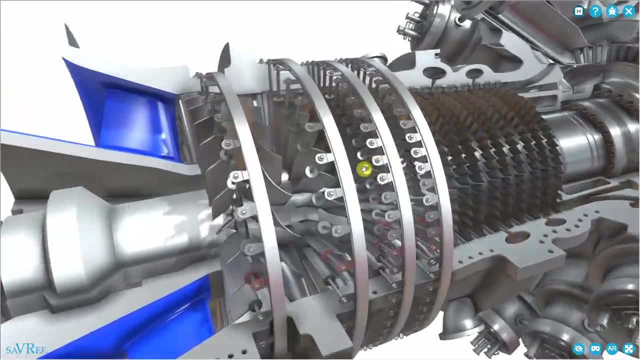 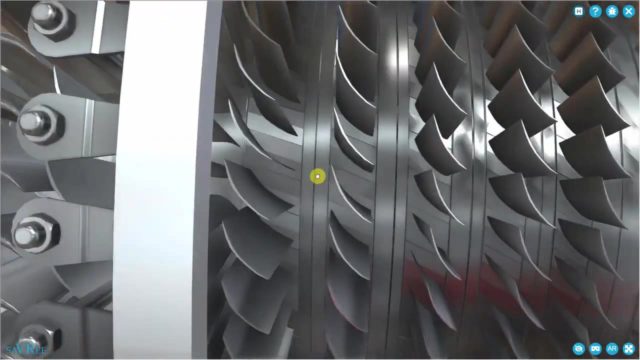 because that's kind of the cool thing about it. It's relatively simple. We've got air that gets sucked in here and the air gets compressed then by a compressor- All of these funky blades starting at about here and moving to the left. 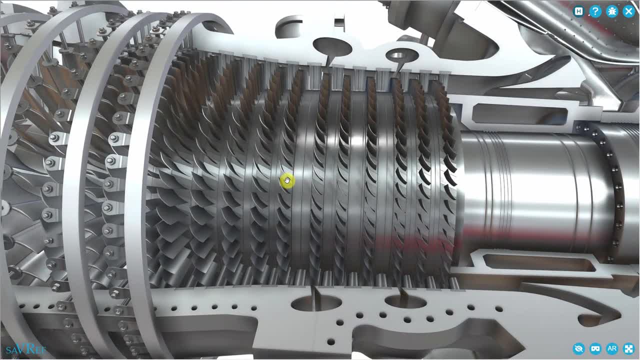 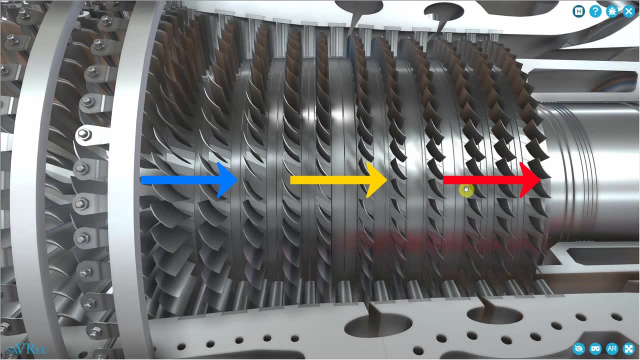 they're all used to compress the air. Each row of blades is called a stage, As the air passes from left to right, as it's drawn in, it's compressed, its temperature increases, its volume decreases, its density increases as well. 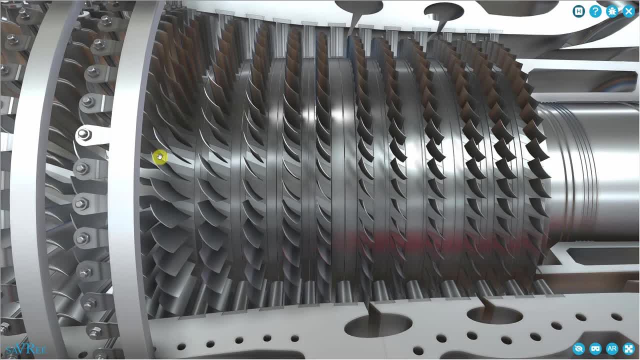 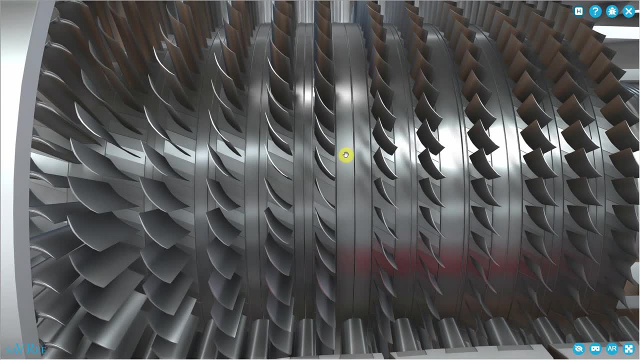 and that's all happening as it moves left to right across each of these stages. So we can have a row of compressor blades and each row is a stage In terms of how much you compress the air. on this, for example, here we are looking at a ratio. 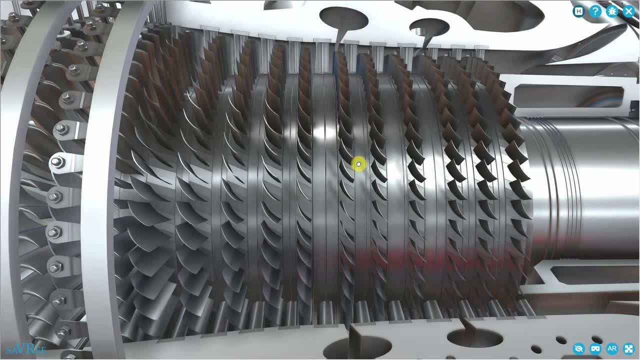 of about 15 or 18 to one. Different types of turbines go all the way up to 30 to one. It depends upon the design. I don't want to go into too much detail, though. This is just a just for fun video. 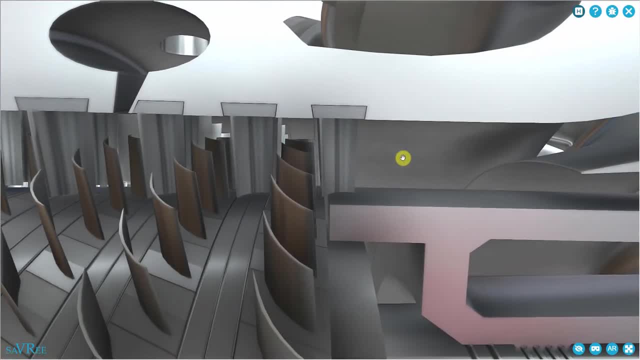 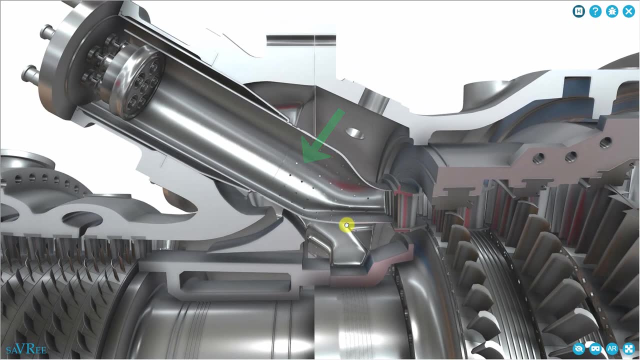 So we're compressing the air, We're then going to discharge it here along and into roughly this space here, and we're going to heat up the air by igniting fuel. The fuel is ignited within this space, within this combustion chamber. 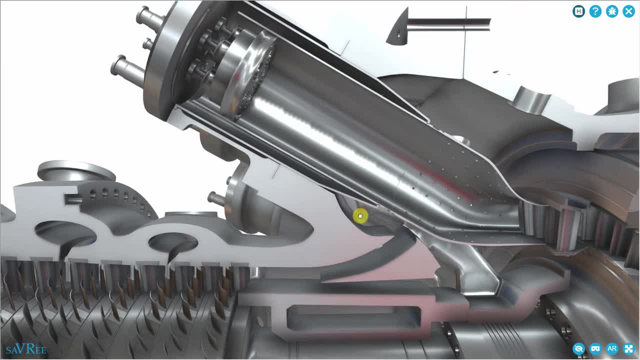 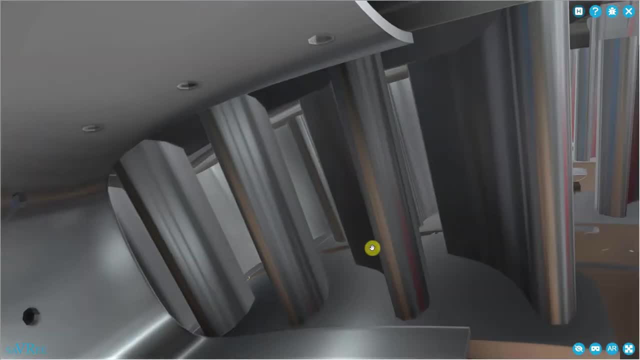 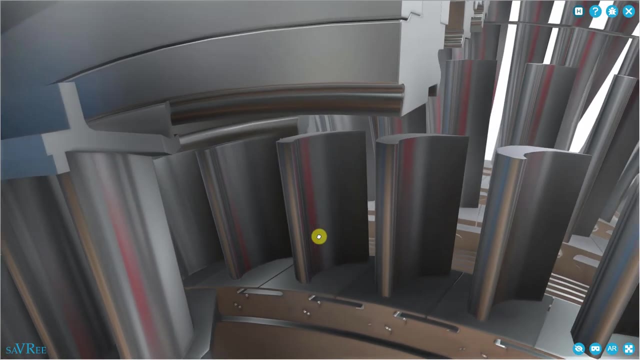 and the fuel then transfers its heat energy to the air. The air gets heated up and then it is discharged through these gaps here, through the nozzles- these are called nozzles- and into the turbine section, So these turbine blades, once we pass the hot gas over them. 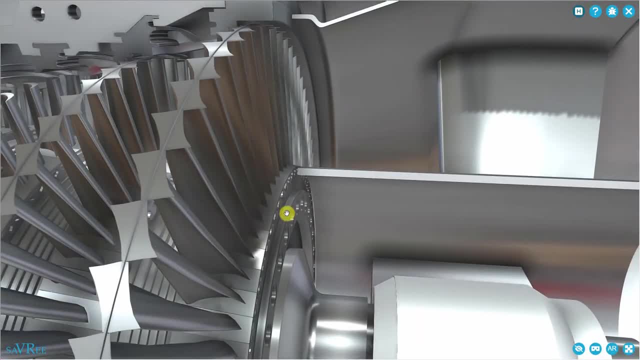 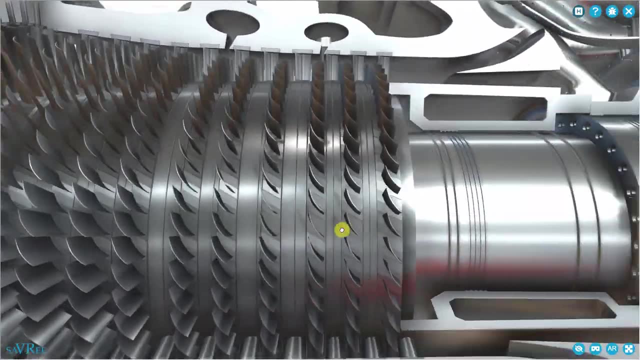 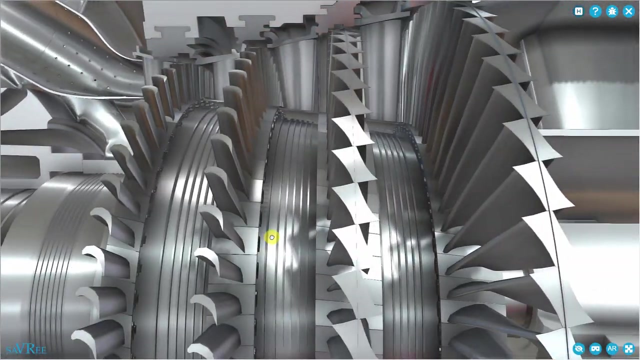 they're going to rotate. So we've got three main parts to the gas turbine. We've got the compressor section here, We've got the combustion area, which is here- Sometimes we'll call this a combustor as well- And then we've got the turbine section, which is here. 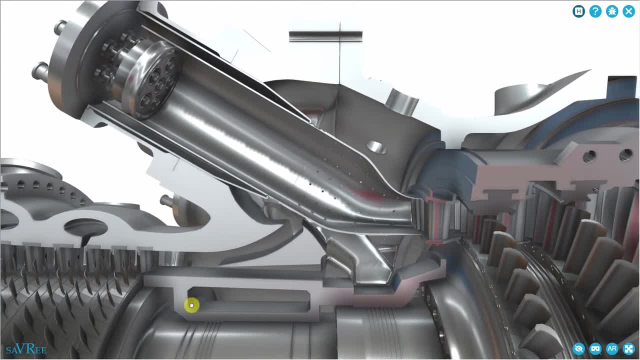 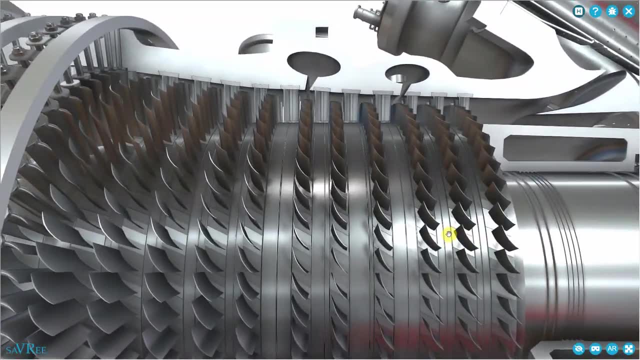 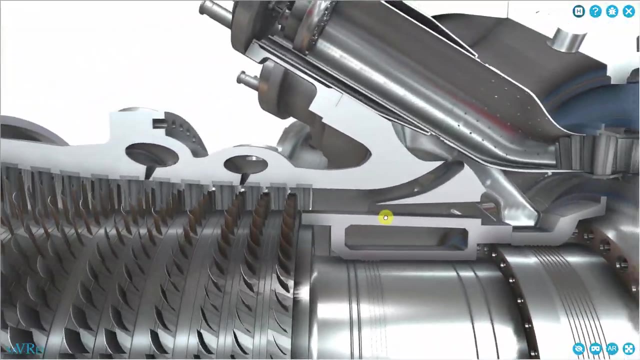 So compress, ignite or combust and then expand. In other words, suck, squeeze, bang, blow. Suck, squeeze, bang, blow. Pretty easy to remember if you remember it like that. I don't know why people say suck, squeeze, bang, blow. 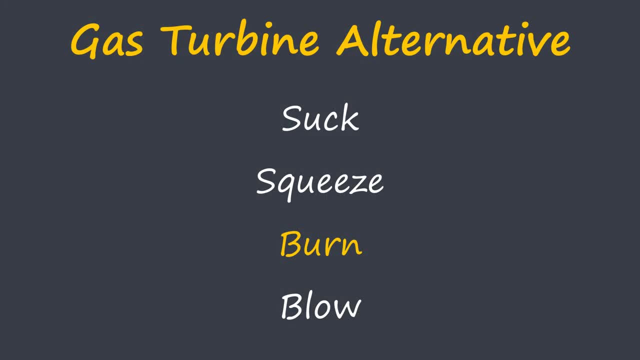 Sounds a little bit weird if you ask me, but I didn't invent the term Either way, though it is quite easy to remember it when you say it like that: Suck, squeeze, bang, blow is also what you do in a combustion engine that we use within cars. 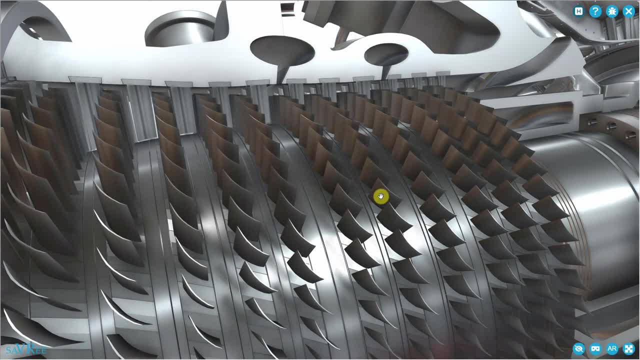 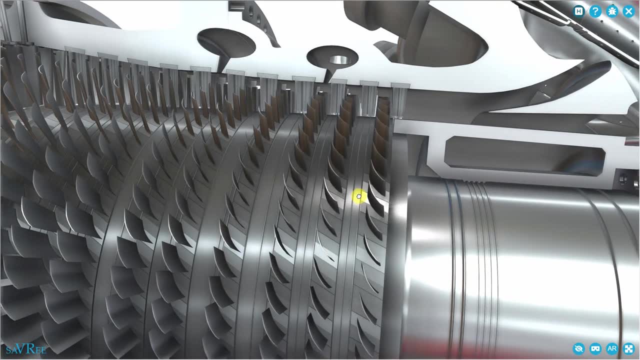 For example, a two-stroke engine or a four-stroke engine: Four-stroke engines for cars and trucks, et cetera, and two-stroke engines more for smaller things like bikes or very large things like ship engines. Either way, though, there are also. 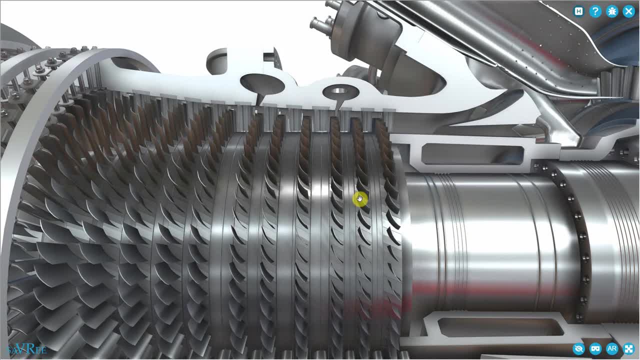 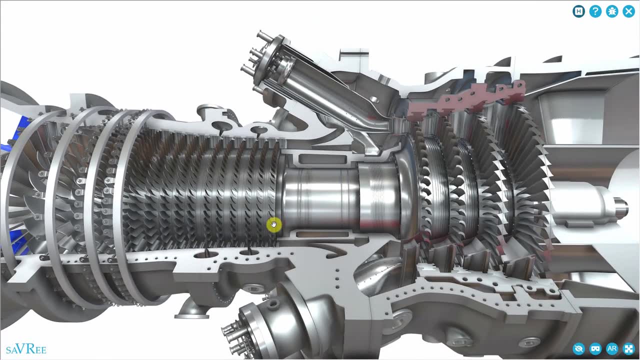 internal combustion engines- the four-stroke and two-stroke engines, and this is an internal combustion engine as well. The difference is, though, this one's actually a constant or steady flow combustion engine, because we're constantly drawing the air in, heating it up and then discharging it. 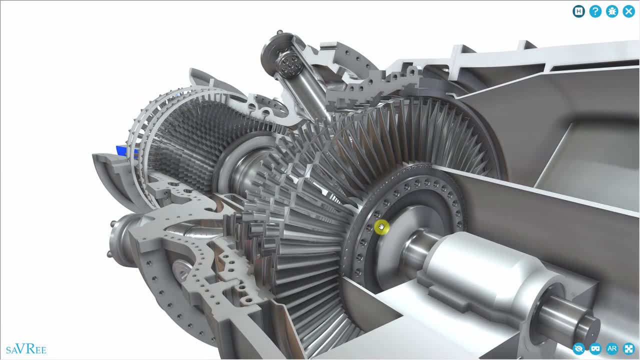 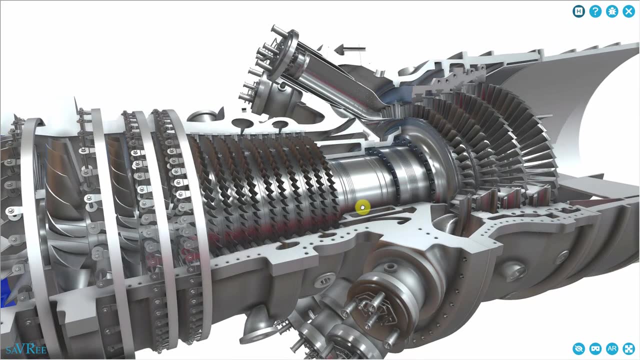 With a combustion engine, specifically the two-stroke and the four-stroke type, combustion is not continuous or steady like it is here, So that's a big difference between a gas turbine or this type of internal combustion engine compared to a two-stroke and four-stroke engine. 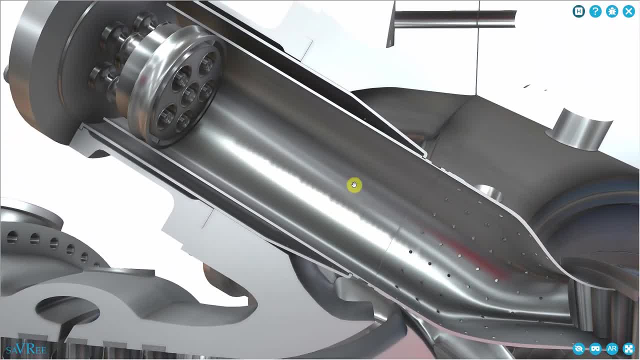 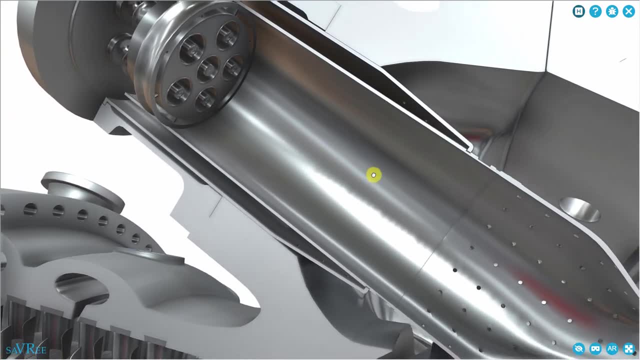 The fuel that's being ignited here. it may be natural gas, it may be pulverized coal, it may be some sort of light fuel oil like diesel. So there are many different things it could be, but it's going to be ignited in here. 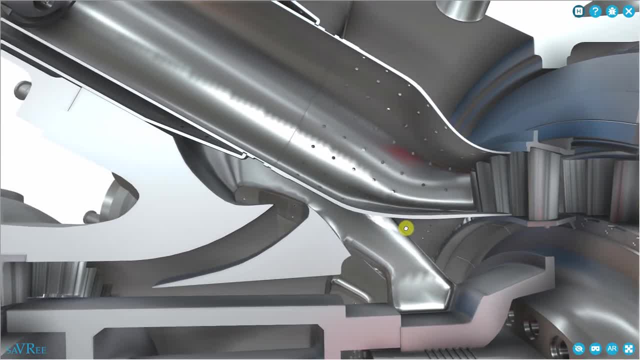 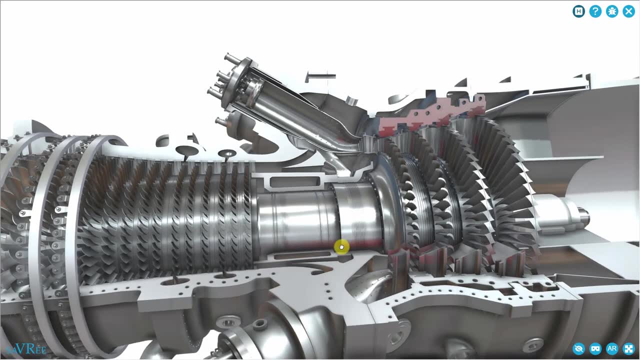 and then we heat up the air and discharge it. We call it a gas turbine. A lot of people believe we call it a gas turbine because it runs on natural gas. That's not actually true. We call it a gas turbine because it runs on gas. 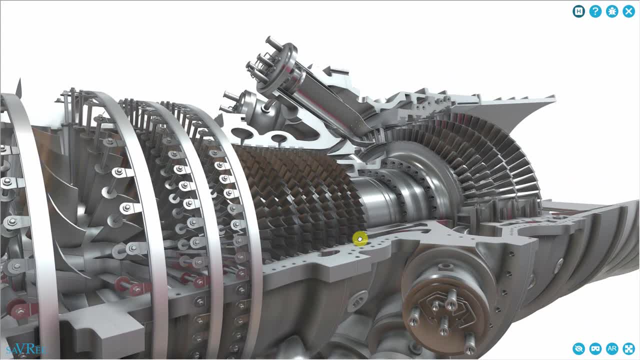 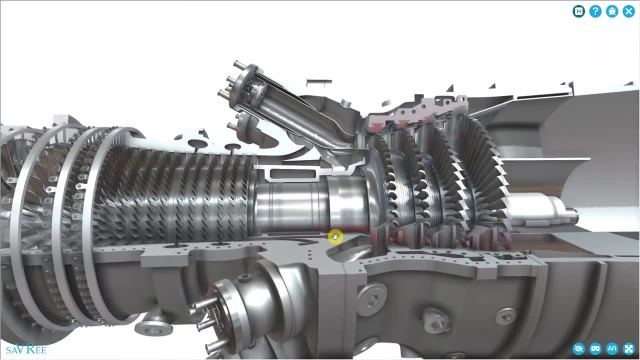 as in a sort of subdivision of a fluid. To really hammer this point home, it's possible to run this turbine on a different type of gas. The gas that we are running it on here is air. We're just sucking the air in here. 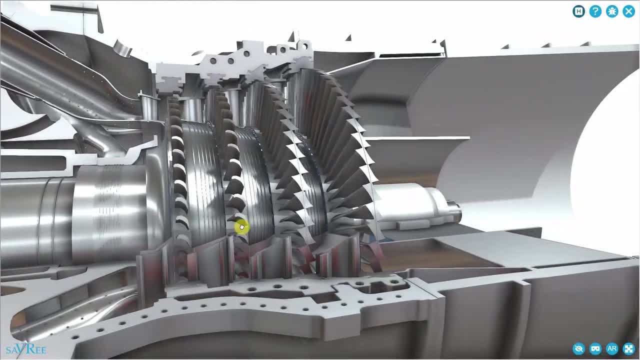 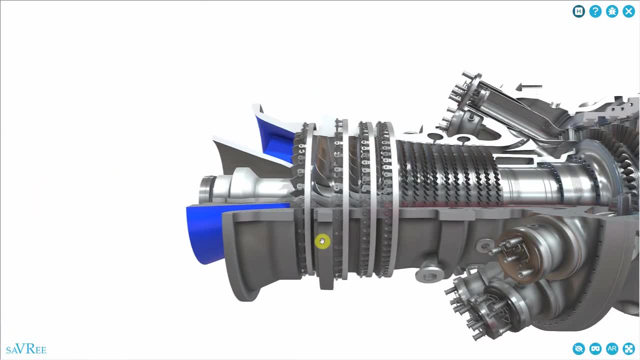 and then compressing it, heating it up and then discharging it. That's what we refer to as an open cycle. But you can also have a closed cycle, gas turbine And what we do: we use a different gas and we'll close off this end. 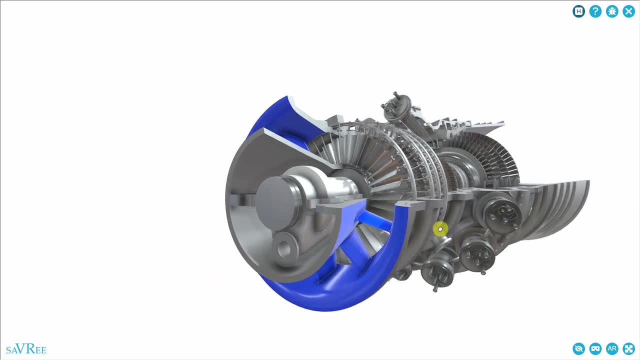 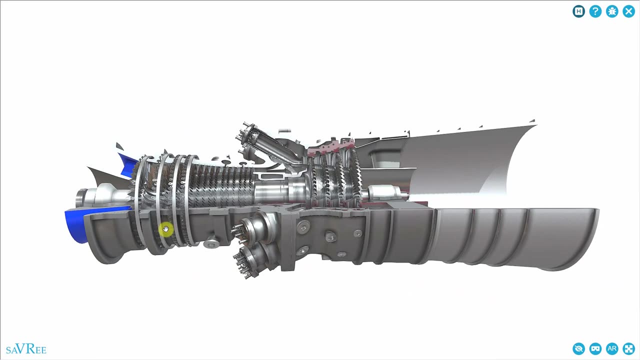 connect it to a bit of piping and then a large tank and we close off this other end here and we'll pass a gas into and out of the turbine and it will just circulate. That's what we call a closed cycle gas turbine. 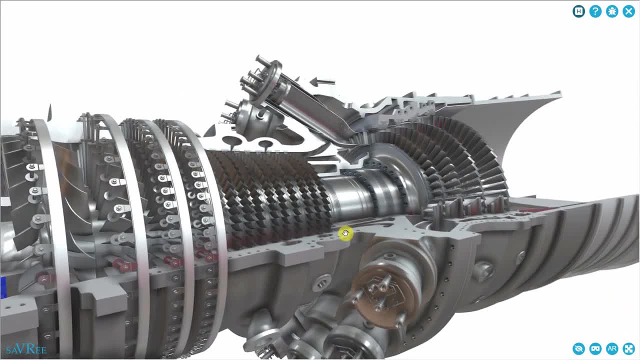 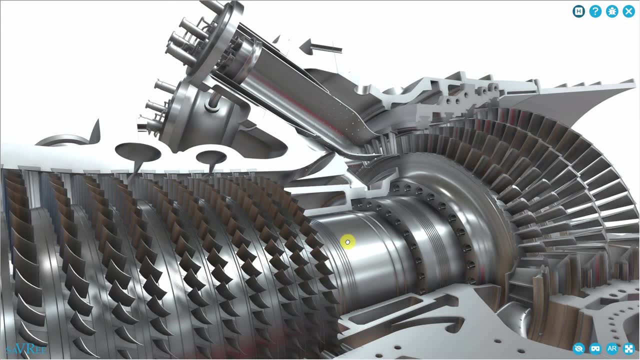 as opposed to an open cycle one. Like I say, though, just because it's called a gas turbine doesn't mean it runs on natural gas. It can be fired on up to around 30 different fuels, Depends upon the design and manufacturer. 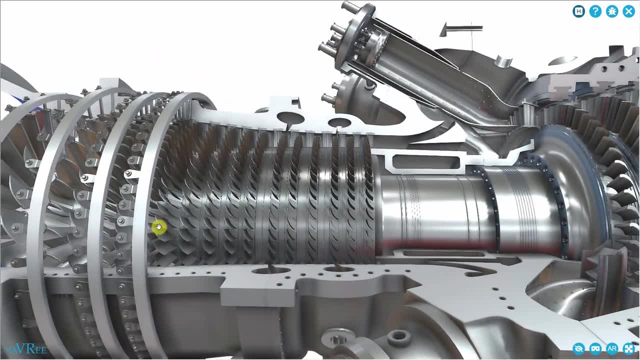 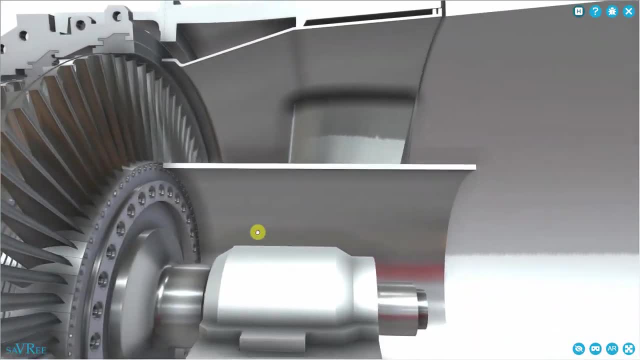 So quite a simple kind of turbine. It's a simple concept: really: Bring in the air from over here, compress it, ignite a fuel, heat up the air and then discharge it over here, And that way we can use a gas turbine. 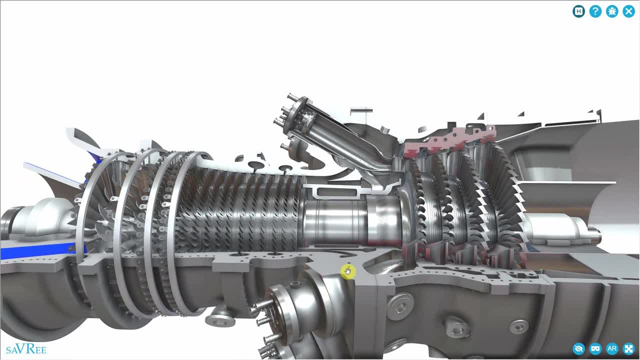 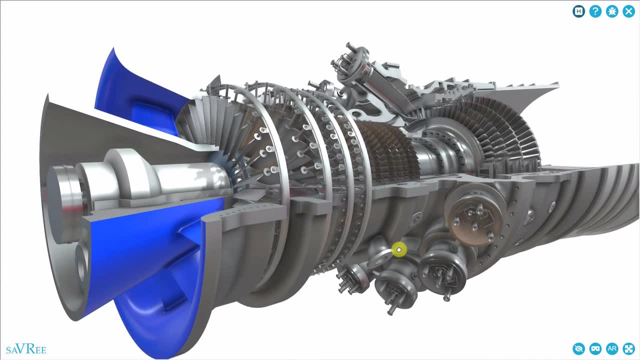 to generate a lot of thrust, for example, for getting an aircraft into the air. We can use a gas turbine for propelling ships through the water, and we can use gas turbines for generating electrical power. That's what this one is actually used for. 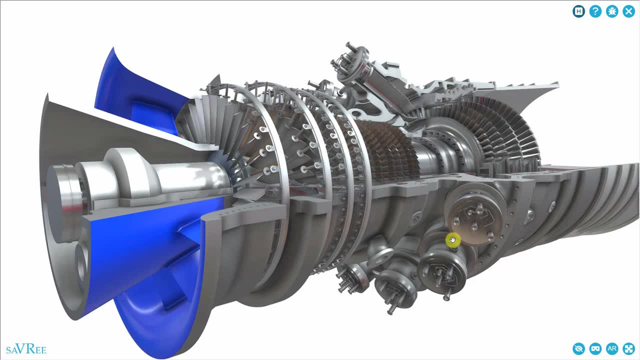 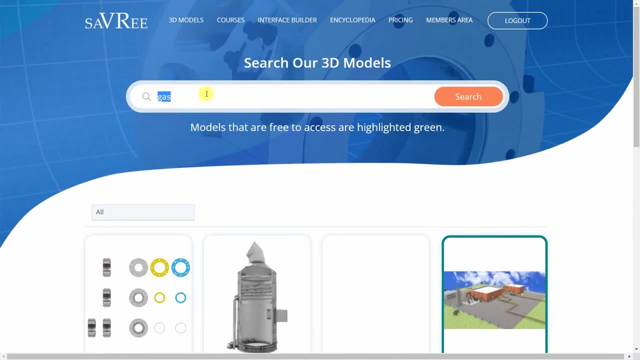 Let's have a look at a type of power station that does use a gas turbine, Because then I can explain to you how that works as well. So here we are again. Let's just have a look, for I guess it's going to be under power station, maybe. 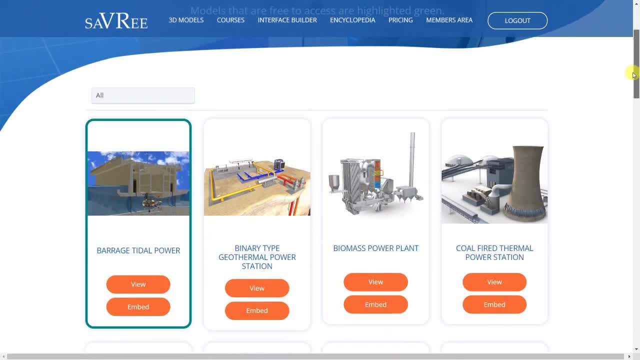 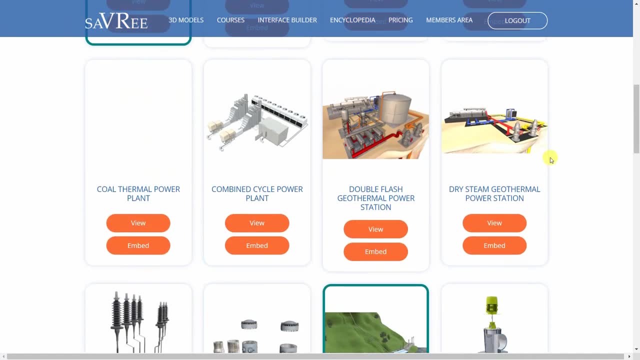 Remember, you can access all of these 3D models as well, if you want to, at savricom, as well as a lot more engineering video tutorials and courses, et cetera. Definitely check all those out if you've got time. 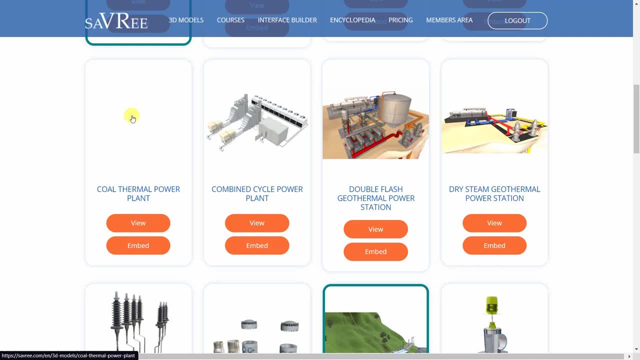 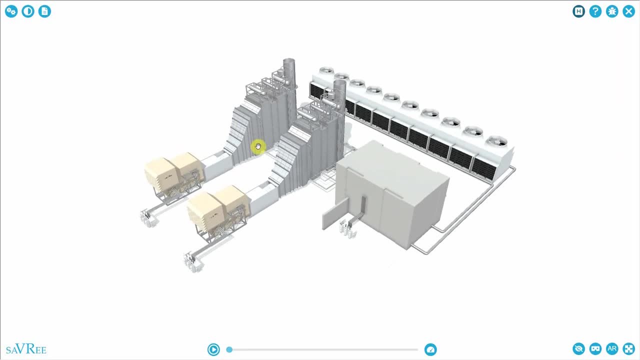 Ah, there we go. Combined cycle power plant. We've got a coal-fired power plant here as well, Also hot off the press, which is why it doesn't have an image. yet Now you're speaking my language. if I spoke engineering. 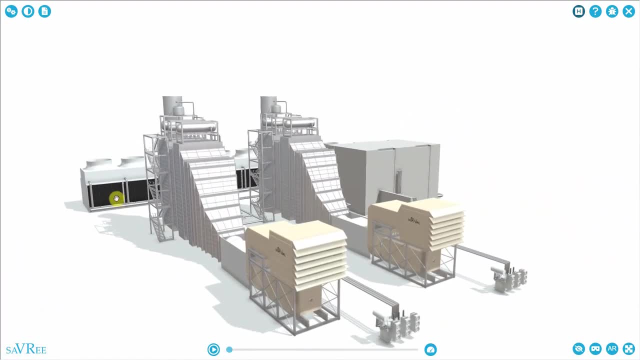 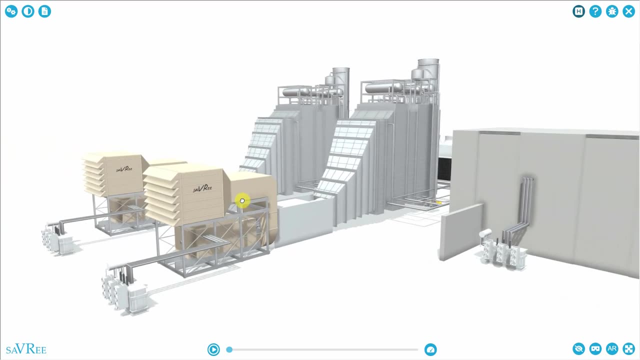 So we've got a power station here. It looks pretty cool. So good job by our 3D artist there, Mo. He's built something pretty cool, as usual. We've got electrical transformers here. These are used for distributing electrical power. 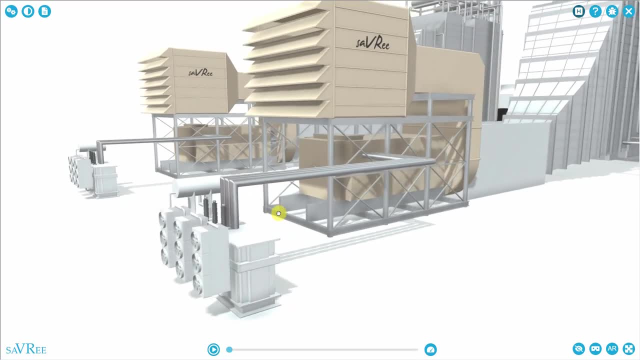 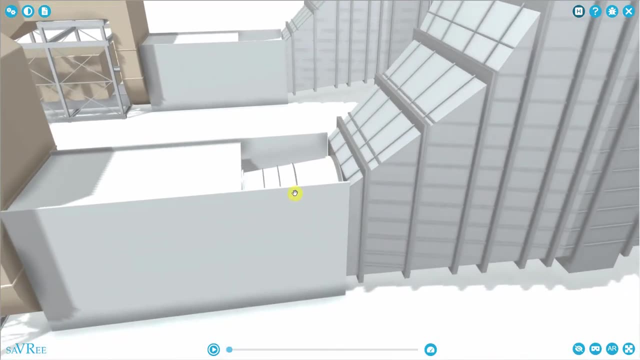 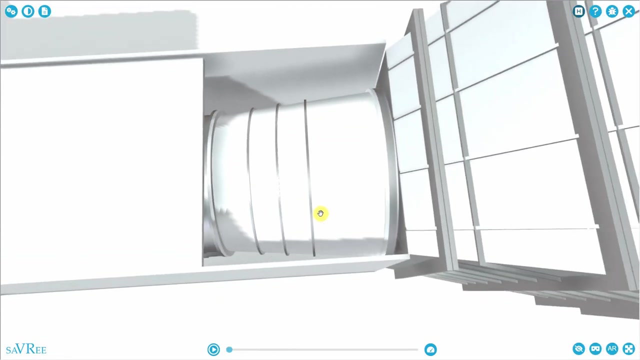 from our power station normally to a substation and then into the grid. Our gas turbine is actually in this box where my mouse is. It's discharging the hot gases here, probably at about 500 degrees Celsius, maybe 550 degrees Celsius. 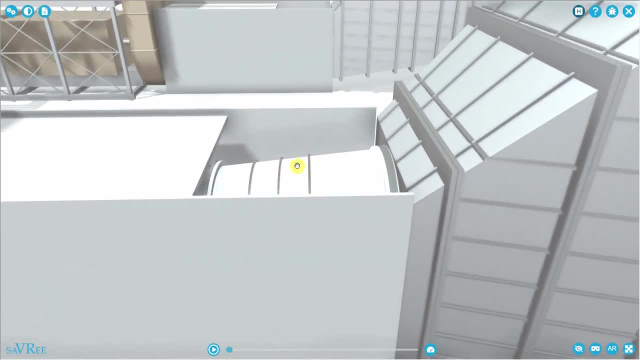 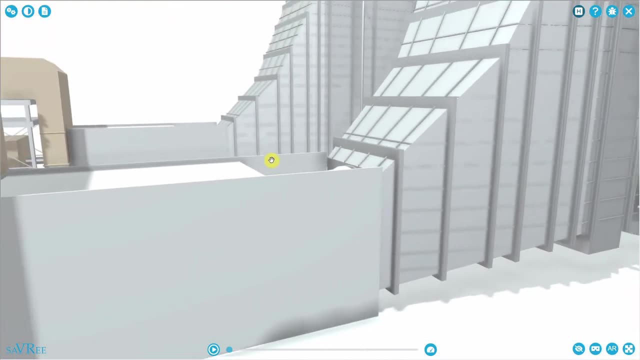 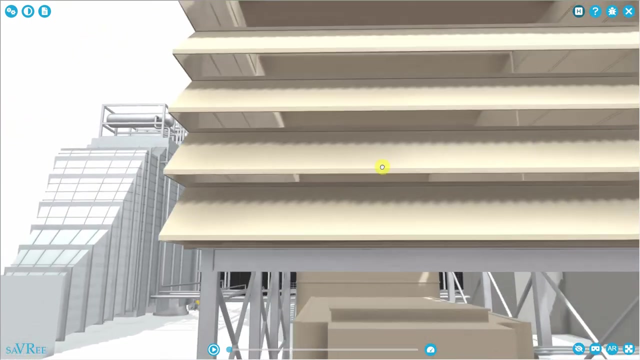 And rather than send that heat straight to atmosphere and just waste it, we're going to use it to generate steam. Before we have a look at that, let's just follow our suck, squeeze, bang, blow theory that we have, So we're going to draw the air in through these levers here. 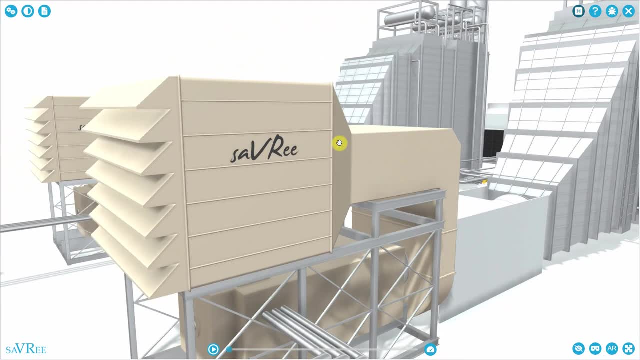 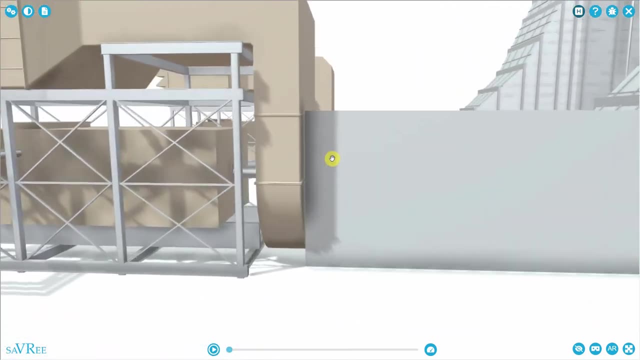 The air is actually going to pass through some filters because we don't want to damage our turbine. when we draw in some air, maybe particles that are in the air, We call these foreign bodies. So the air comes down along here, down into the gas turbine. 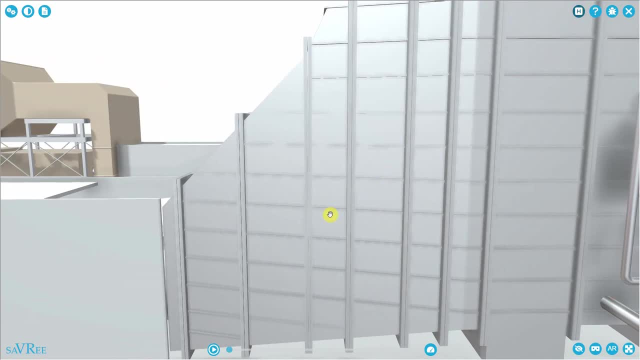 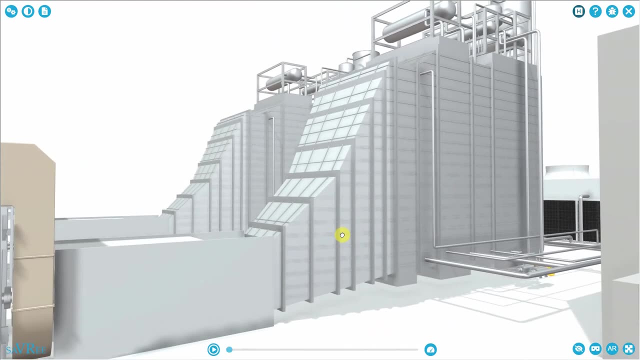 and then we heat it up and discharge it into this item over here which looks like a massive piece of Lego or something similar. It's actually called a heat recovery steam generator- HRSG- and it's a pretty interesting piece of equipment as well. 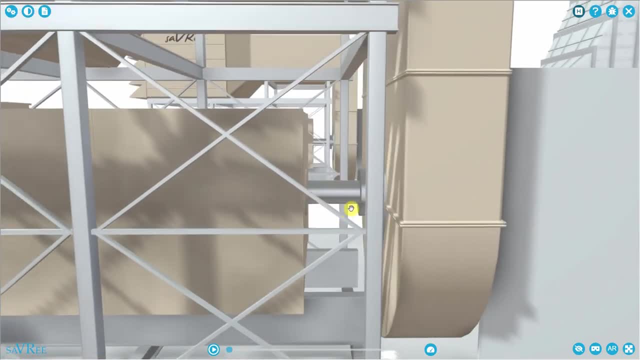 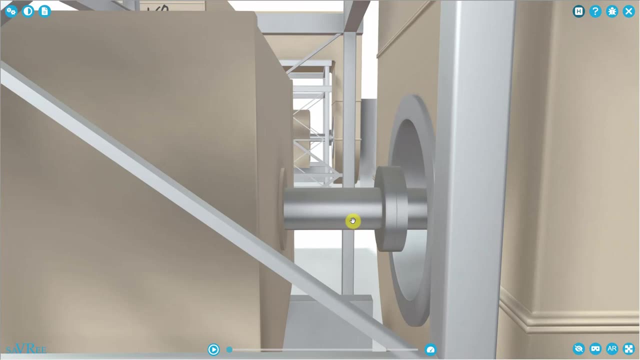 We'll take a look at that in a sec. The gas turbine is rotating so there's hot gases are passing across the turbine. Turbine blades move. That causes the shaft to rotate. We connect that shaft via this coupling here to another shaft. 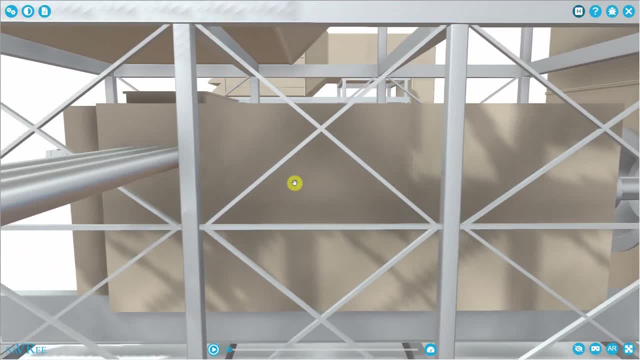 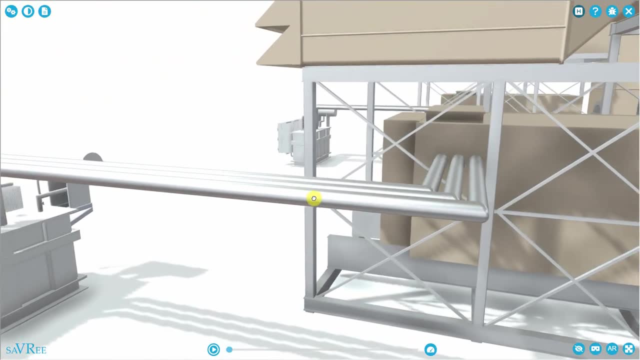 That's our generator shaft. We've got to generate a rotor within this generator box That rotates, we generate electricity, and then we've got three phases of electricity here which we can send to our electrical transformer. Now what do we do with that hot gas turbine? 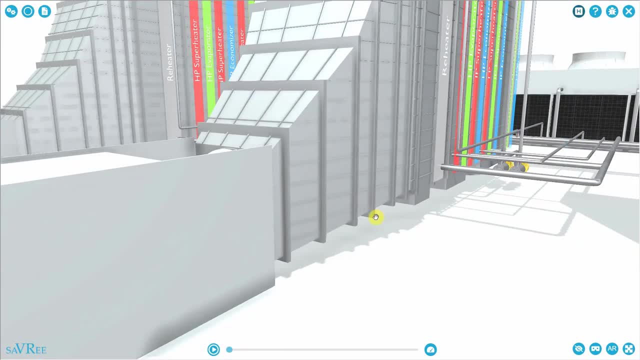 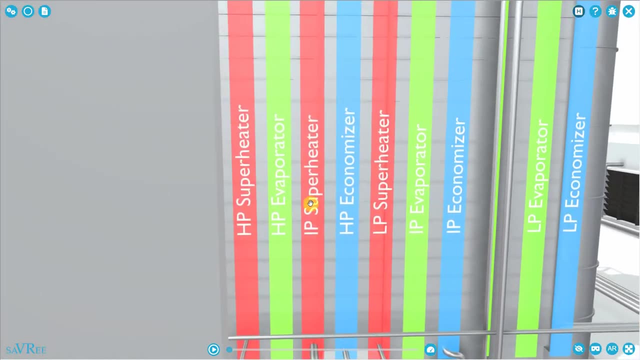 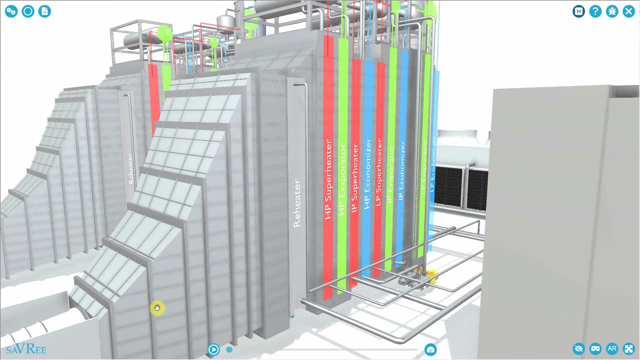 That hot air. we send it out from left to right into our Lego block and it goes into this item here which is called a heat recovery steam generator, HRSG. It's basically a boiler, So the hot gases they'll go in and they'll run. 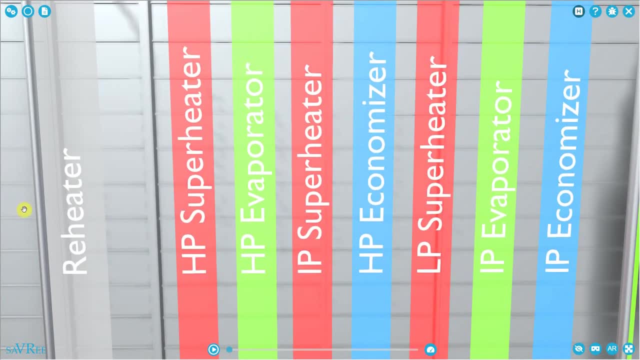 Let me see if I can angle this correctly. They'll flow from left to right across our reheater, across a high-pressure super heater, a high-pressure evaporator, An intermediate-pressure super heater, a high-pressure economizer, a low-pressure super heater. 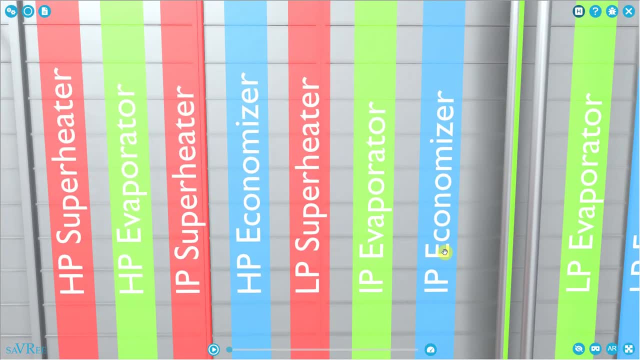 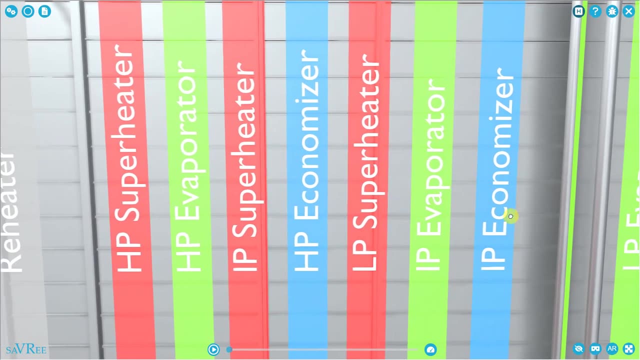 an intermediate-pressure evaporator, an intermediate-pressure economizer, a low-pressure evaporator and a low-pressure economizer. Okay, that was pretty long-winded. It kind of took me a while to get through there, but we got there in the end. 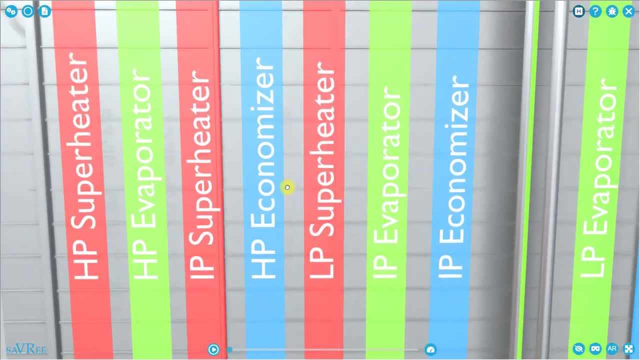 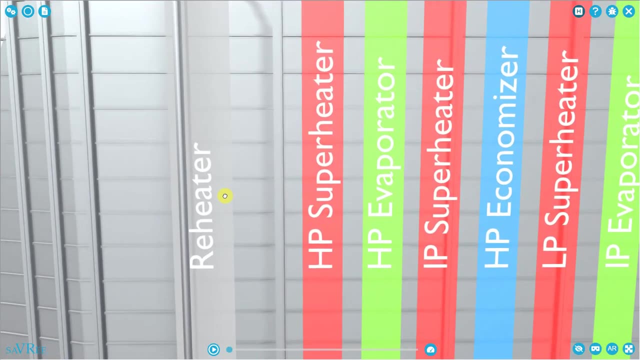 Notice that we've got the economizers in blue, We've got the super heaters in red and the evaporators in green. The super heaters are on the left because that's where the most amount of heat is. The gases are coming from the left to right. 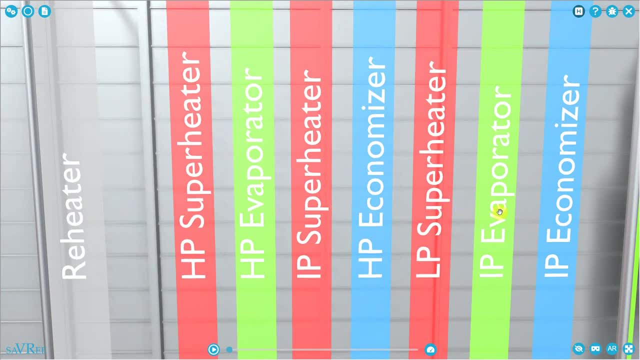 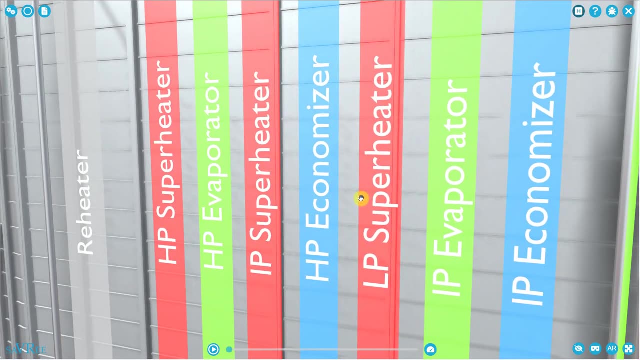 As they flow across each of these items. these are essentially tubes that are suspended within the big Lego box. The tubes are full of water or steam, and the heat from the hot gases is then passed to the water or the steam, and that's how we can generate more steam. 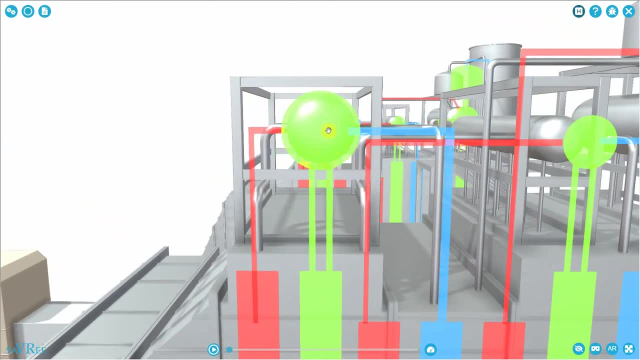 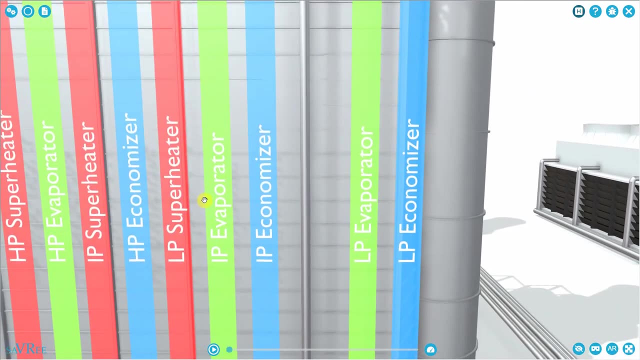 or increase the temperature of the water, et cetera. See, here we've got a steam drum, another one here, another one here, and by the time the hot gases get all the way over, here you can see that they're funneled. 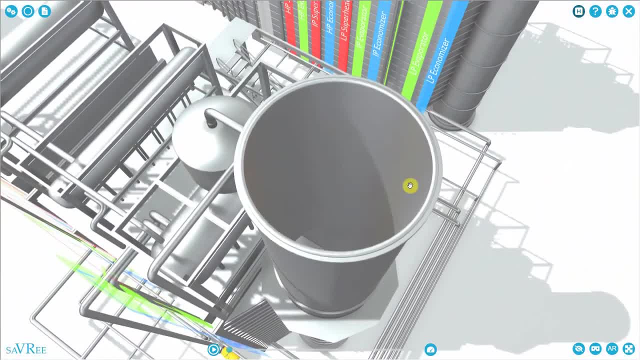 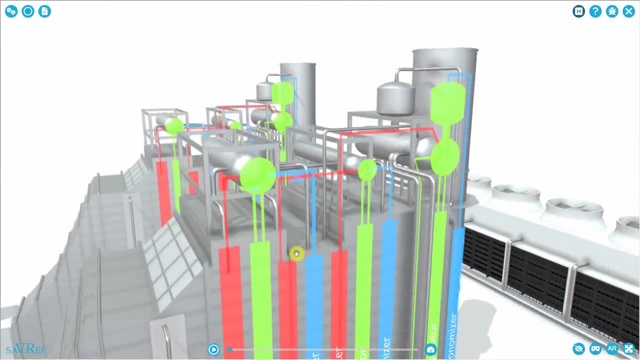 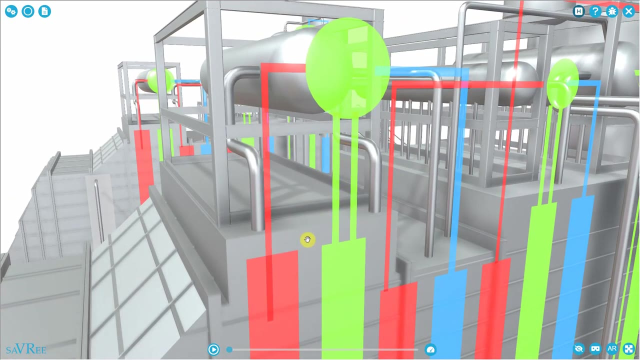 towards this circular stack, which some people call a chimney- I call it a stack- And then the hot gases flow out of the top of the stack. So by using all of these tubes, you can see some passing here, here, here, et cetera. 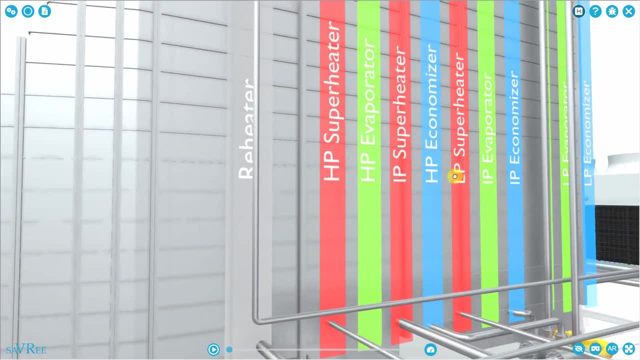 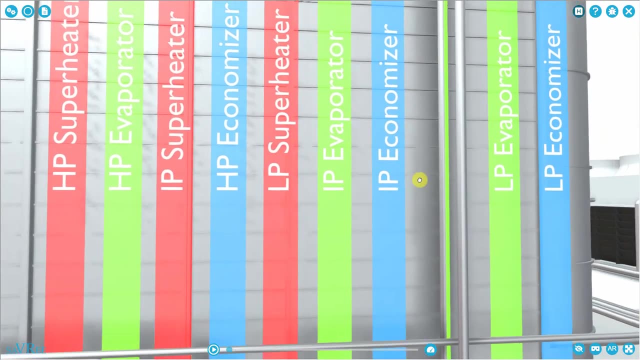 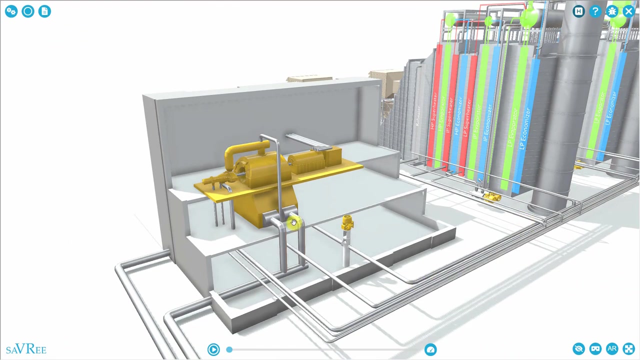 By using all the tubes and putting them within the heat recovery steam generator, we can actually create steam. We can actually create steam because otherwise we would have just wasted the heat from our gas turbine. We then send the steam. see, it comes around here, along here and along there. 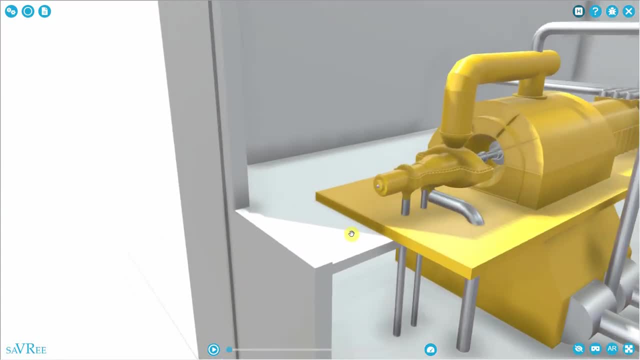 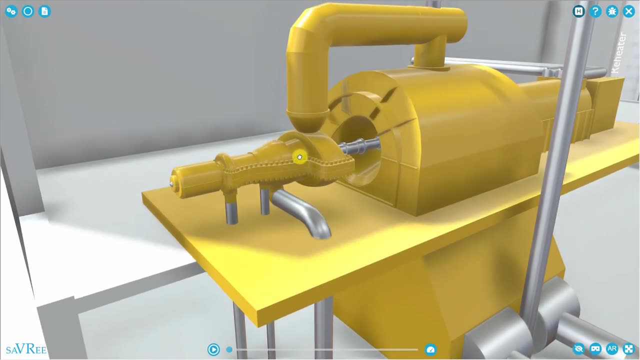 Actually it's coming down here and along here and into this section of the turbine. This is a high and intermediate pressure turbine and the steam turbine rotor is going to rotate. The low pressure steam turbine rotor, which is within this box here, is also going to rotate.